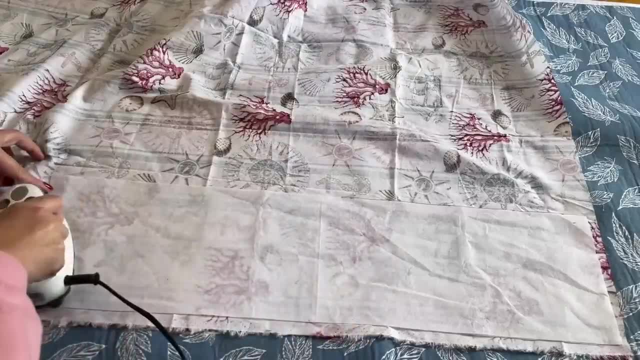 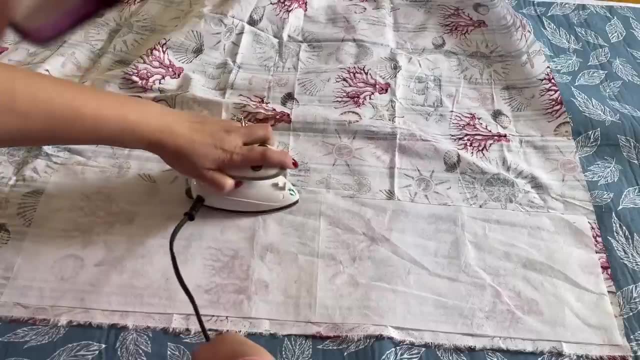 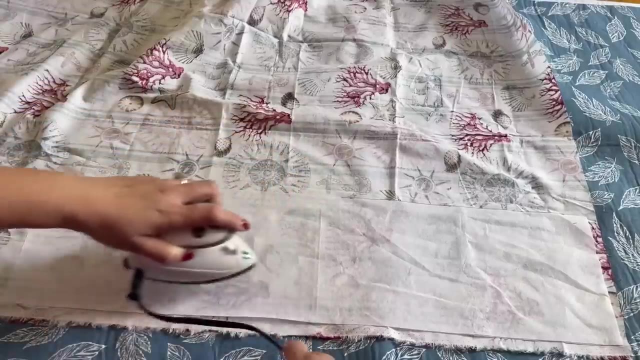 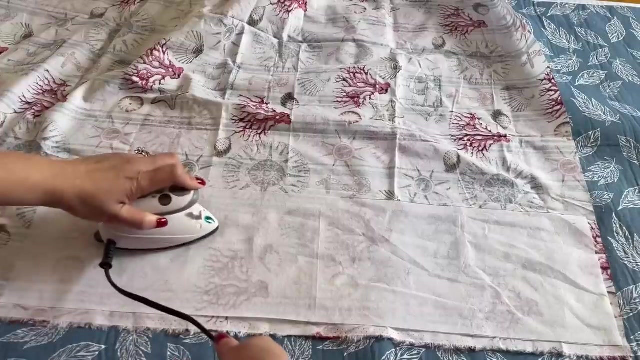 And also make this bubble. I have some kind of side effect from one of the vaccines I have- Not the COVID, no Something else- And it gives me a chill headache and fever for almost a week. The headache is nothing compared. 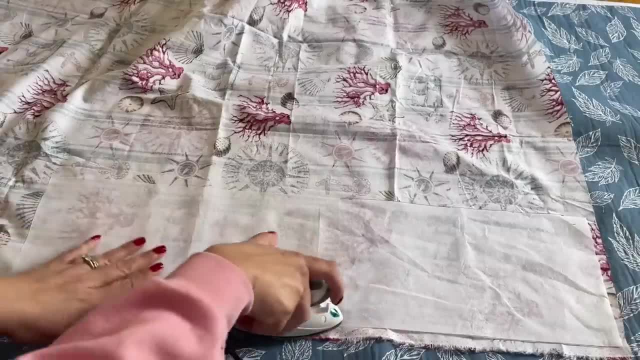 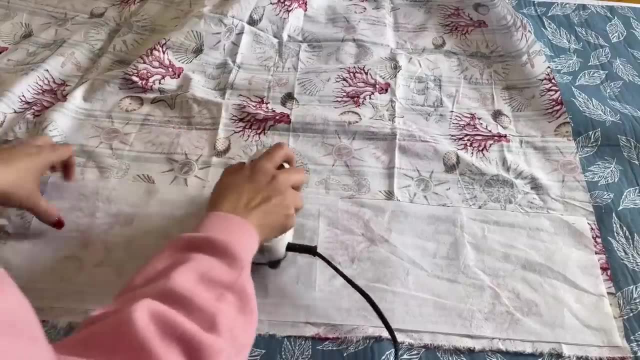 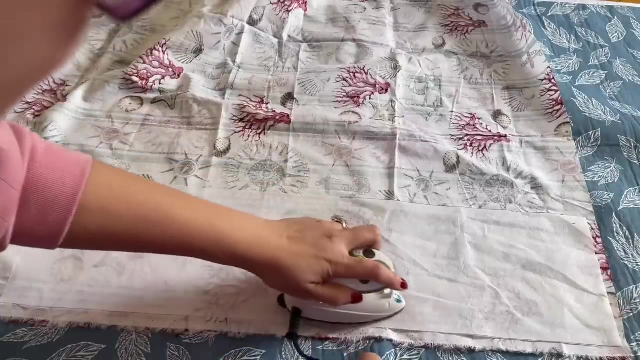 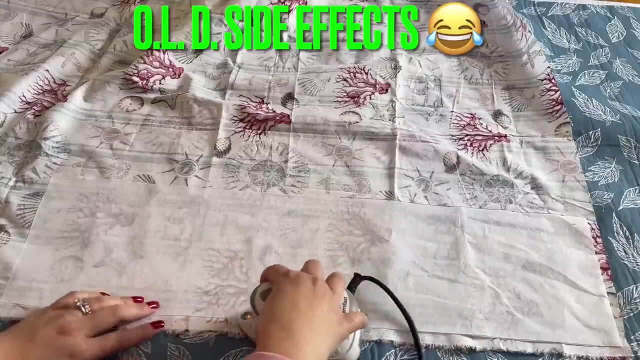 It's so bad. So just get over that. I am alive. And I told my son I'm like I don't know why I have this side effect so bad. I don't know what kind of side effect is this? He said in the back of the car and he said I think you have OLD side effect. 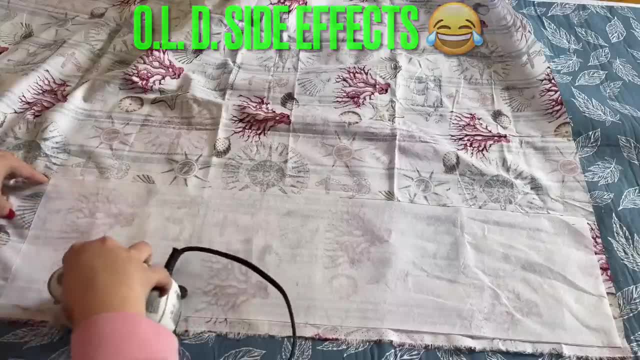 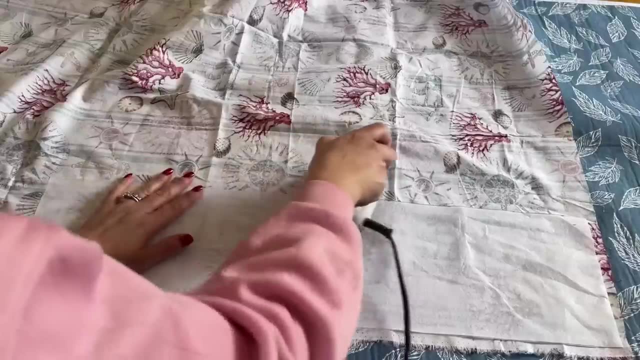 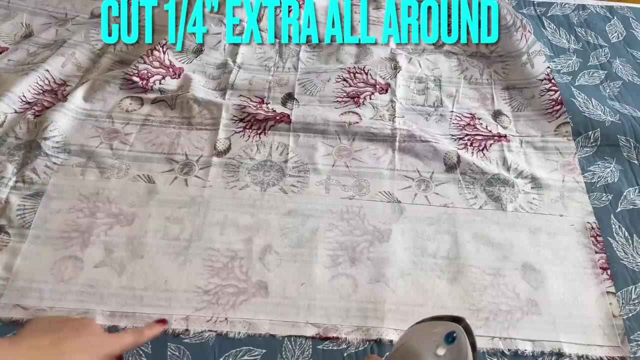 I'm like, what is that? I wasn't thinking? I'm like, what is that He refused to say And I finally got it. I'm like, oh, my goodness OLD, I'm going to go around and cut like a quarter of an inch or around. 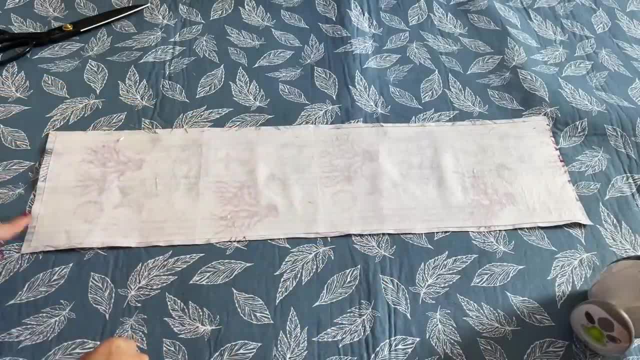 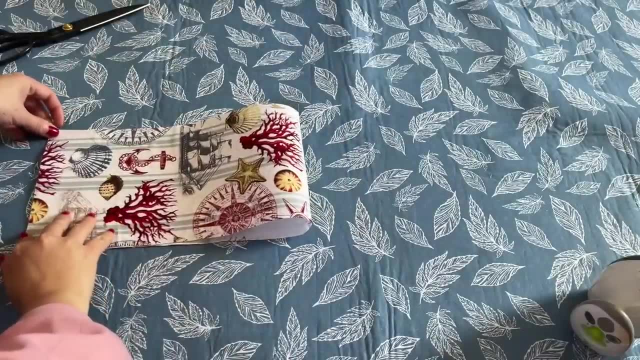 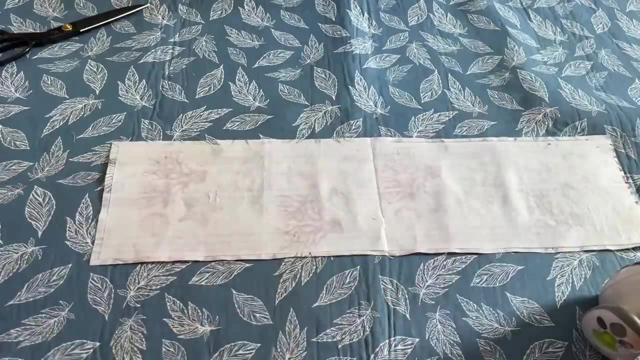 So then, after you're cutting a quarter of an inch or around, you're going to fold it in half, Make sure everything meet up, Just a half- the center line right there- And then open this up. you're going to bring the half. let me just mark it down so you can see right there. 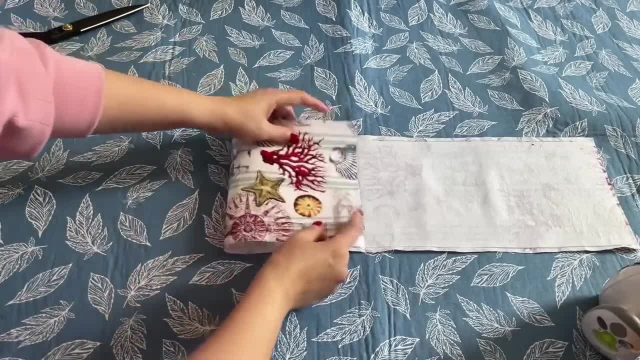 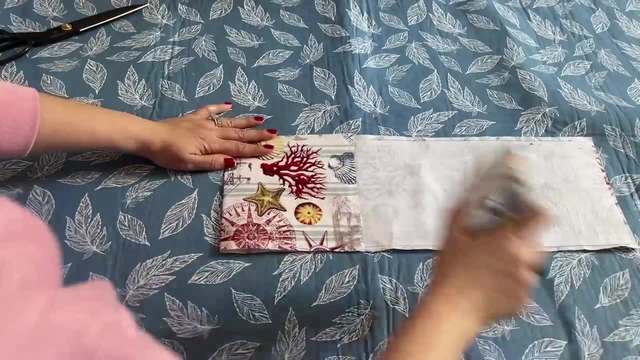 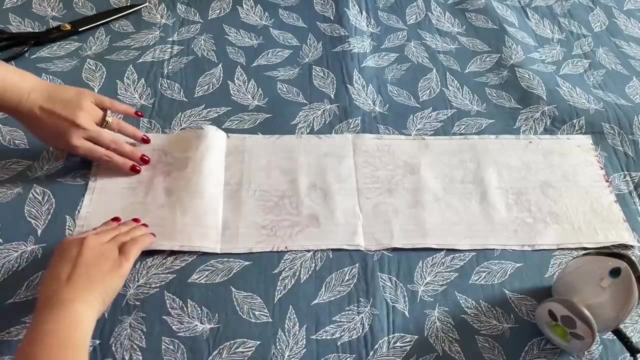 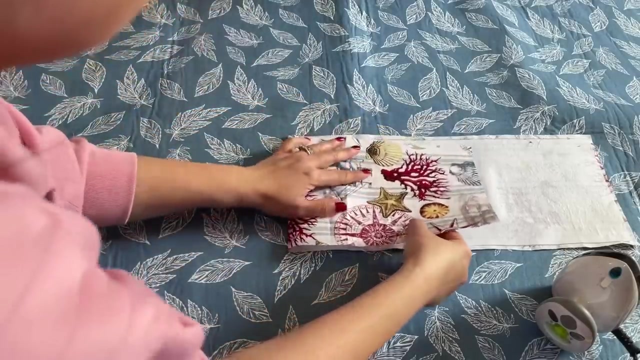 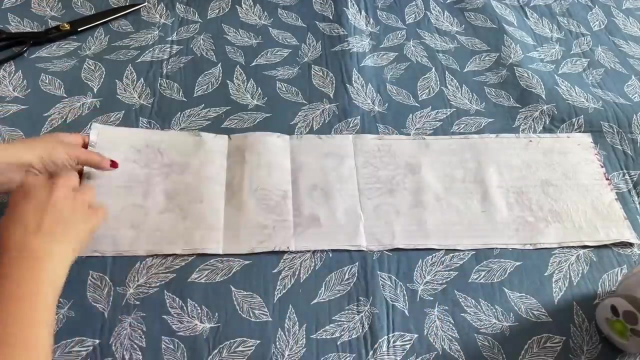 That's the half. So then you bring this half into this, Iron this down, Then you have two, And then you bring in each half here into half, So you divide it into four, Iron this down And that you have two. 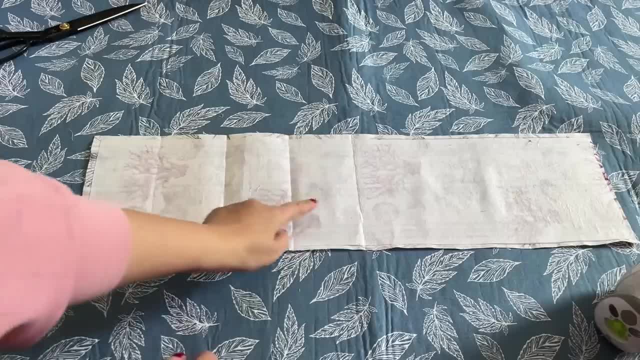 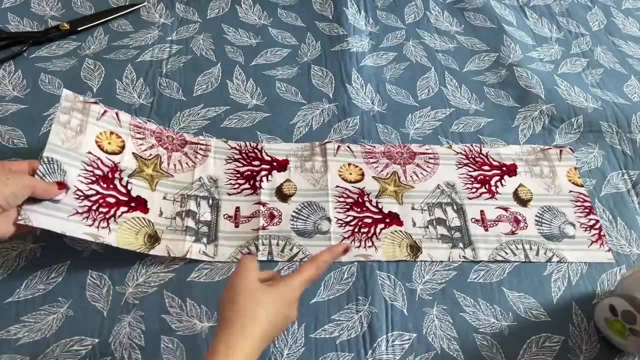 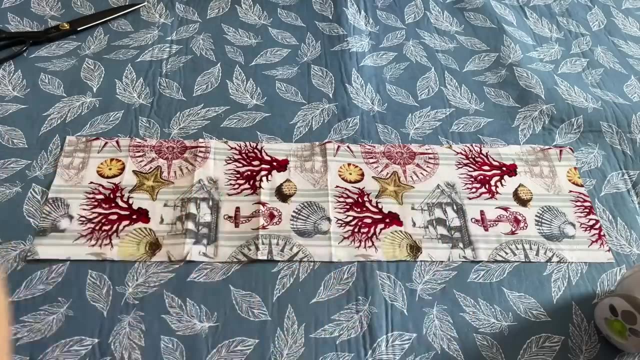 And then this one, you have another one, Two, three, four, And then the other one is half. One thing I just want to share with you: when you cut the fabric, I have the fabric going this way. So when you do, you always have to make sure that you're cutting the way the fabric go. 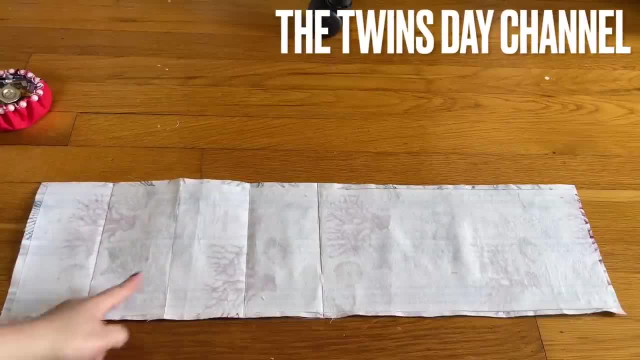 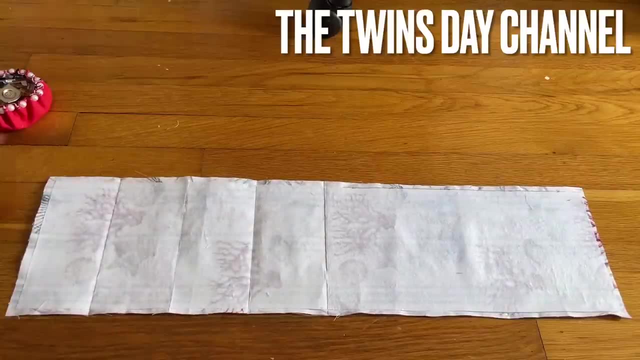 Okay, So every one of the you can I mark here so you can see the four. If you don't want to, you can just get this and then snip on the side, but you don't really need to. Now. the folding is very important. 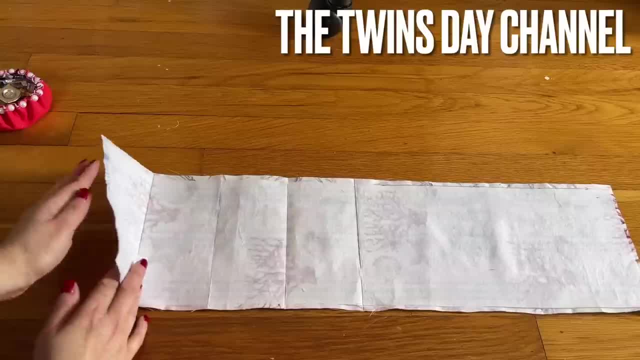 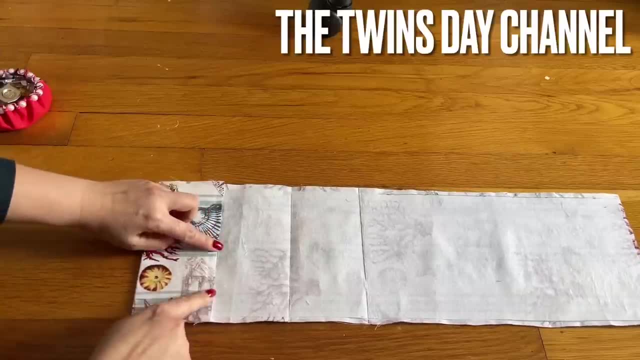 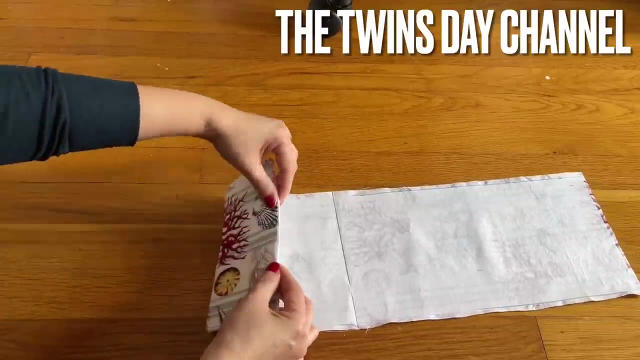 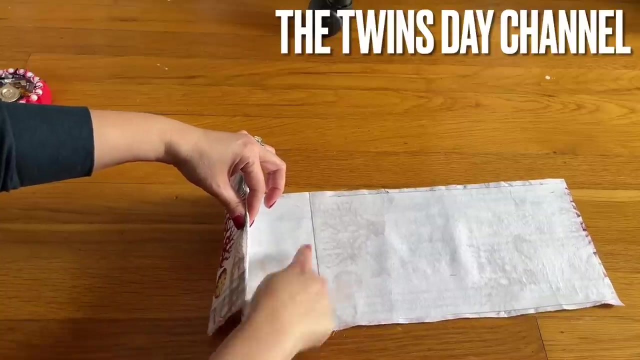 So you go on, the first one on the left, you're going to fold it in, Make sure everything is lined up, And then the second line, the second one right here. you fold it out This way, You fold it out, and then you're going to bring this to the center, the half. 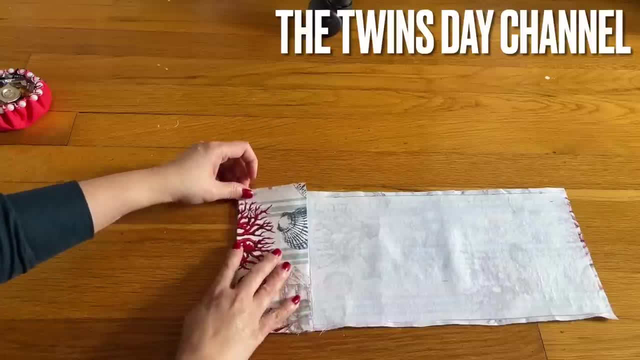 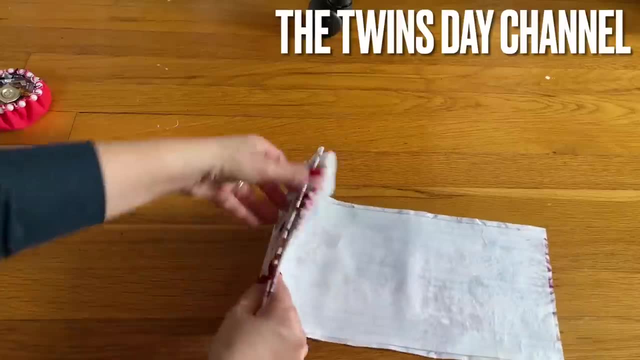 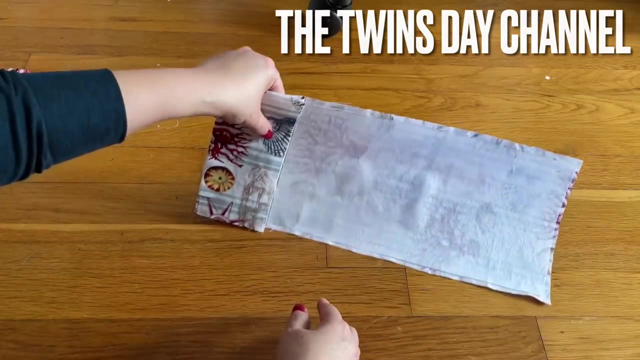 Right there. When you do that, you're going to make sure everything is lined up for you, And now you can see the opening in here, And then here you have the two fold on the left, So just like that, And then you're going to turn into the right. 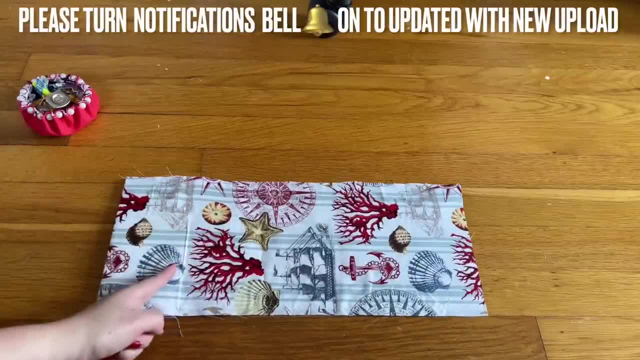 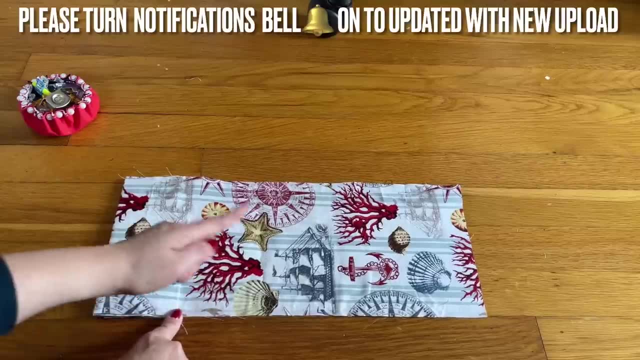 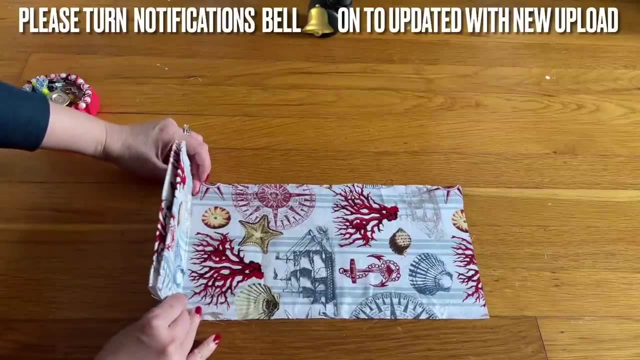 Right side. this way, after you turn into the right side now you can see this is the half, and this is the half that we already fold. I like you to fold in this one right here for one more time. So the line right here. you put your hand right there, you put your finger right there and flap this in. 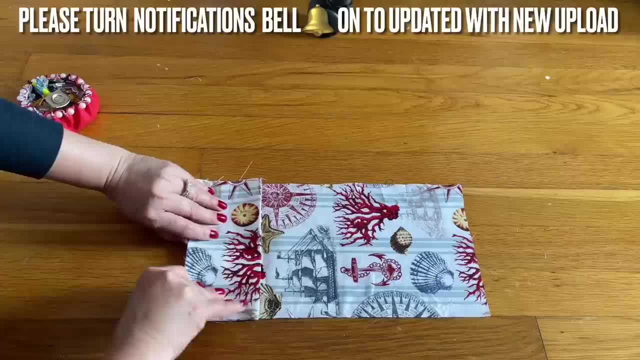 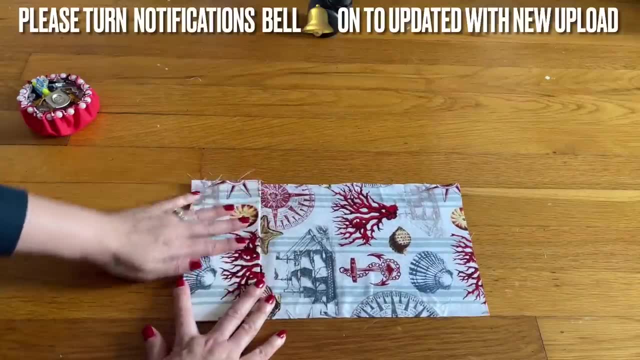 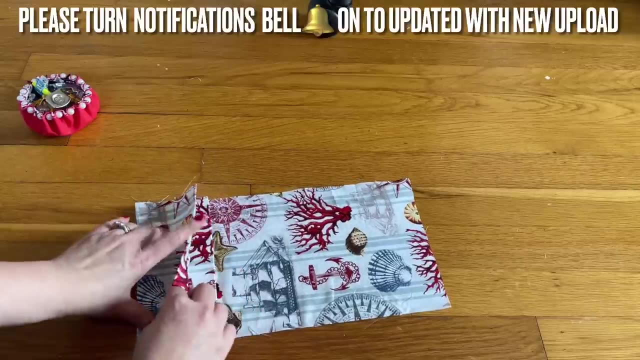 You're going to do one more fold and you're going to make sure it meet up the line that you marked the center earlier when you divide in half. Perfect. Now you can see, here you have the opening and two fold. and then here you have perfectly, two fold. 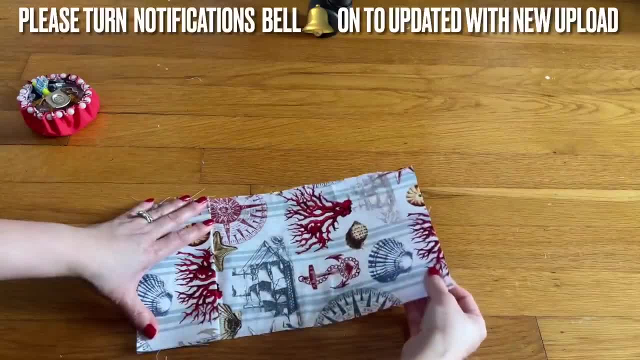 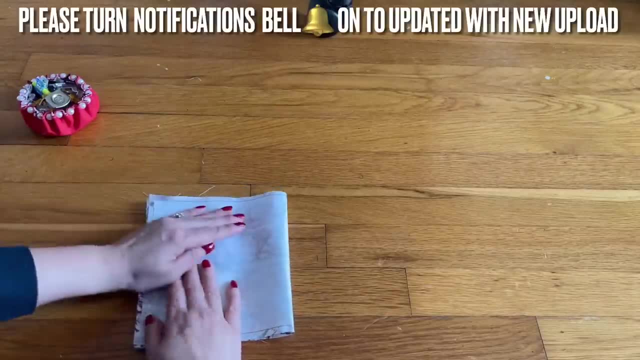 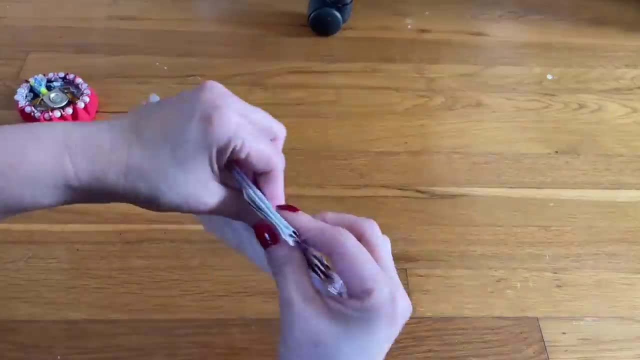 Okay. So now you're going to bring this end over to meet over here. You're going to make sure everything is lined up nicely for you And now you can press around here. Now the reason why I left it a quarter of an inch. 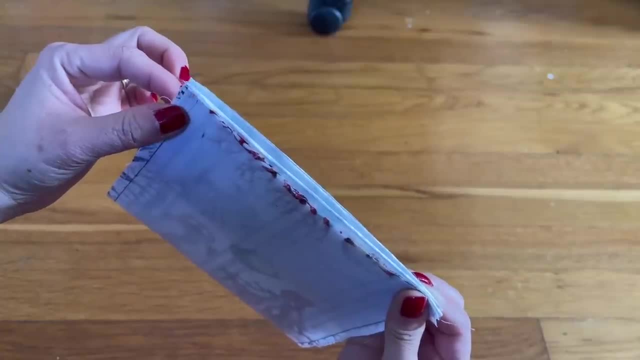 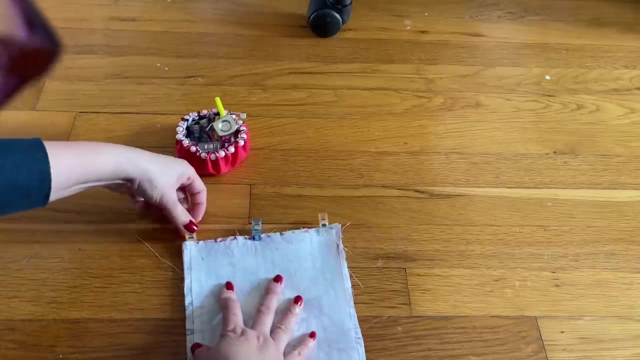 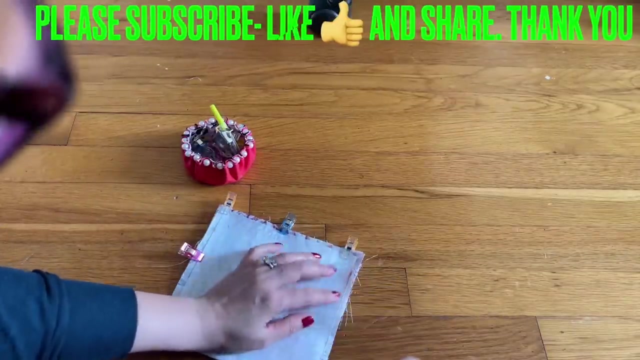 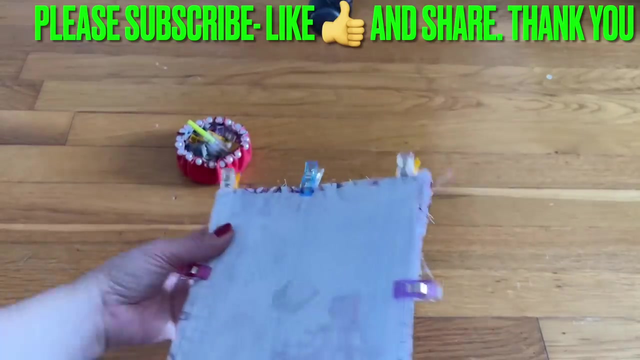 Okay, Here without the interfacing, because I don't want it too thick when I sew. Now you can see we have something like this: Okay, And this is all that fold and the craziness up there, and it's here Only one fold. 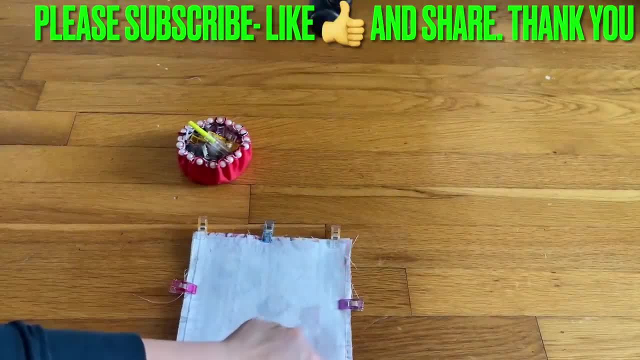 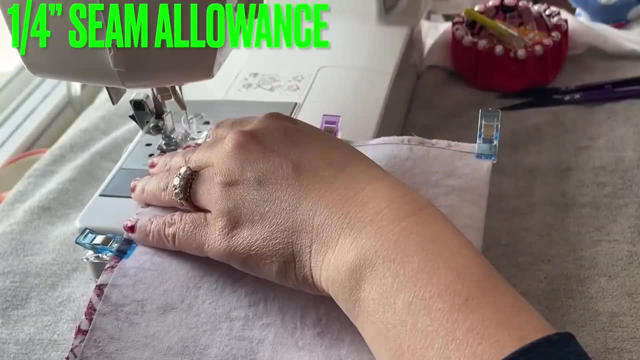 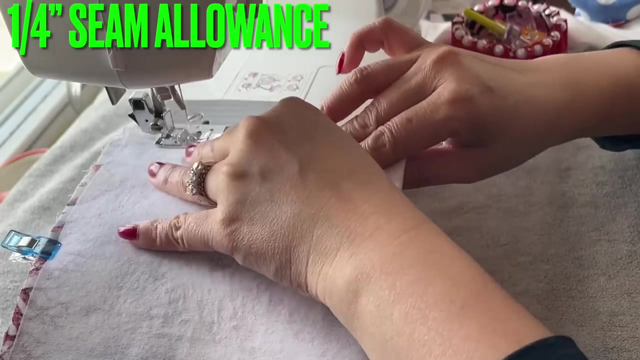 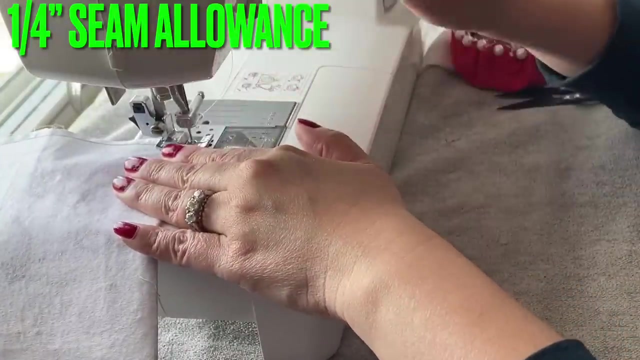 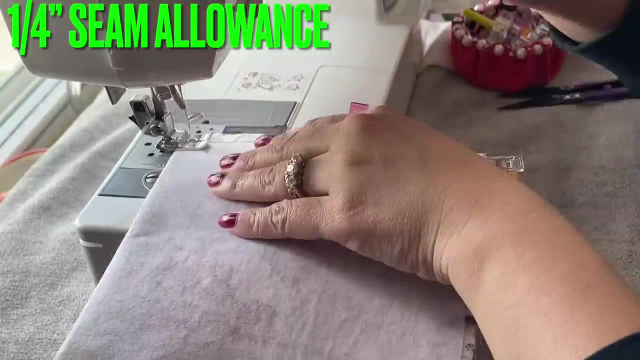 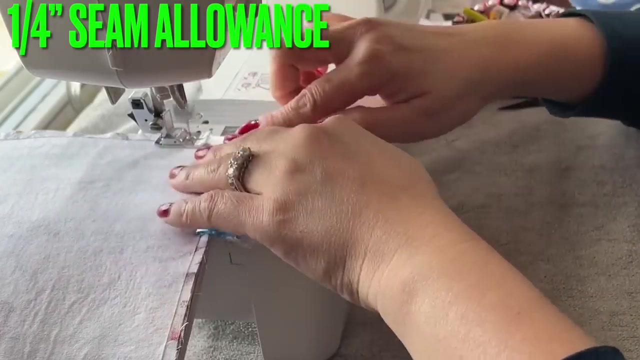 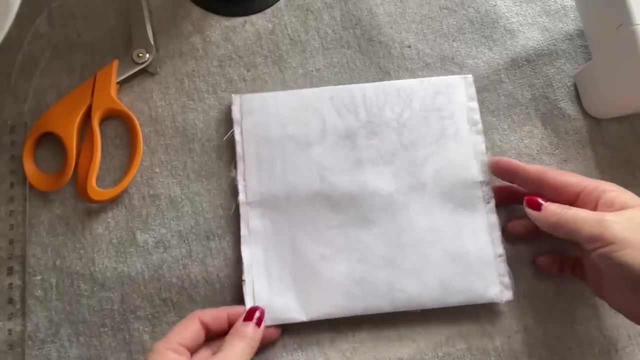 You're going to sew a quarter of an inch and sew this straight line down, This straight line down And then this straight line down. Thank you, Now you can see with the interfacing if you don't do the quarter openings on each side. 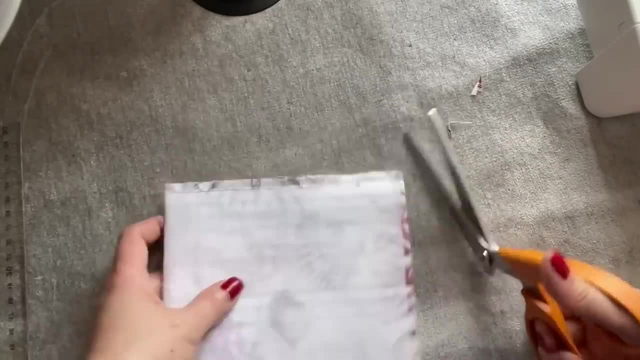 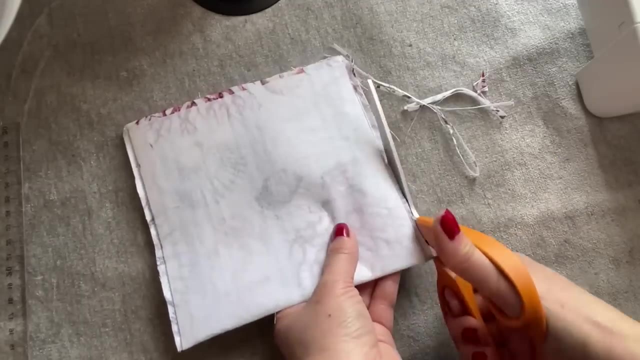 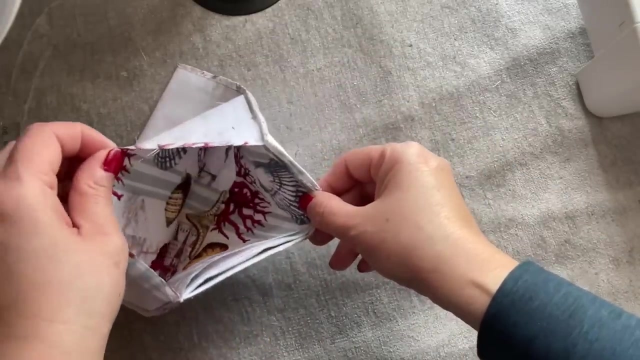 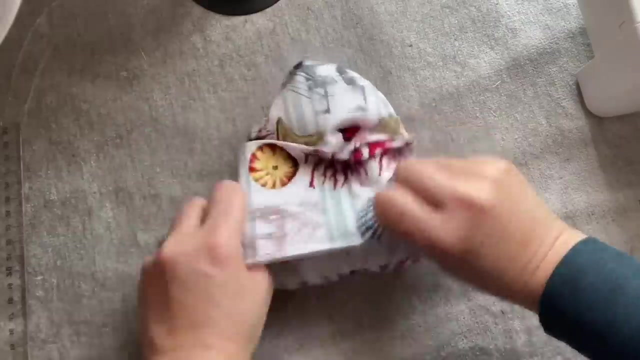 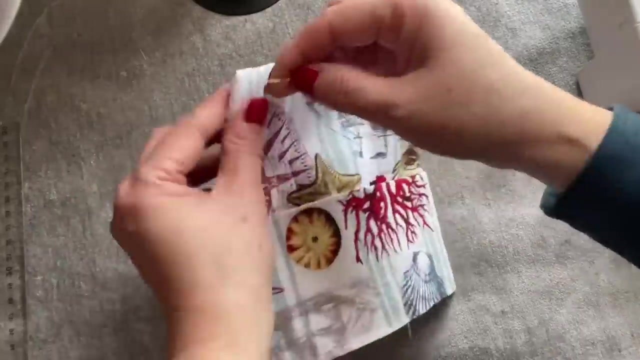 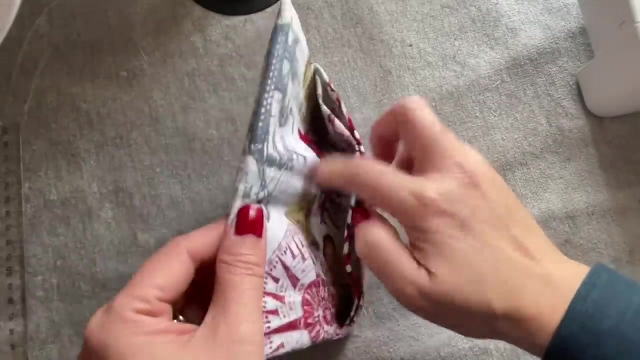 they're going to be so thick for you to sew. Right here on the top we have the opening: Go inside, Inside and inside out this thing, And now you can see we have something like that with the tooth And then the big one right here. 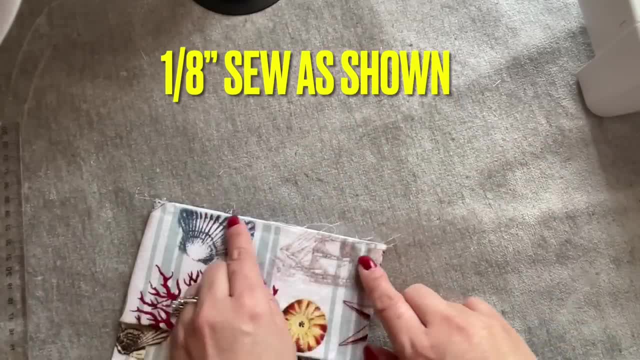 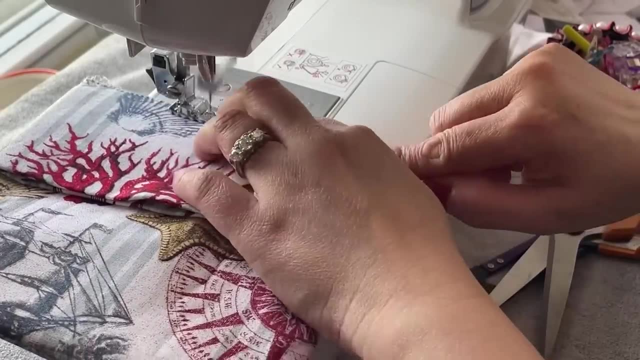 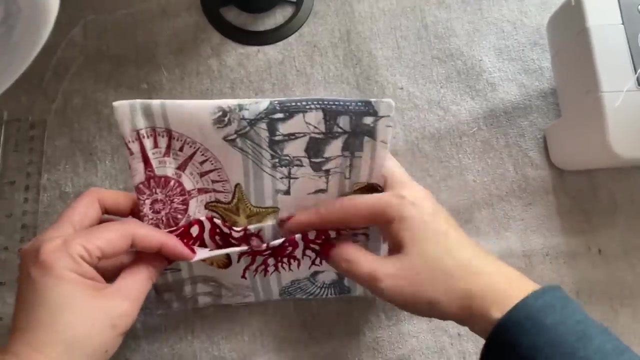 If you want, you're going to be very close on the bottom here and sew this line. So now, when you're finished, you can see the two folds like this, If you hold like this and then you go on to inside out this part, 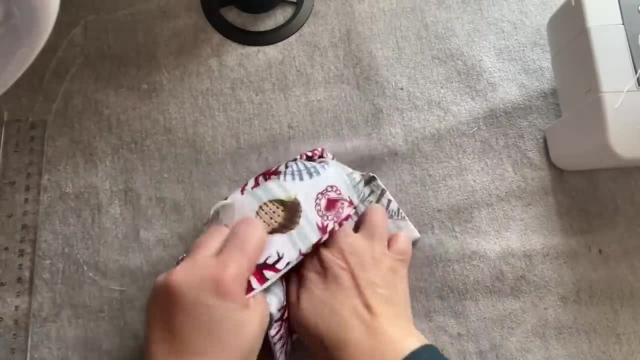 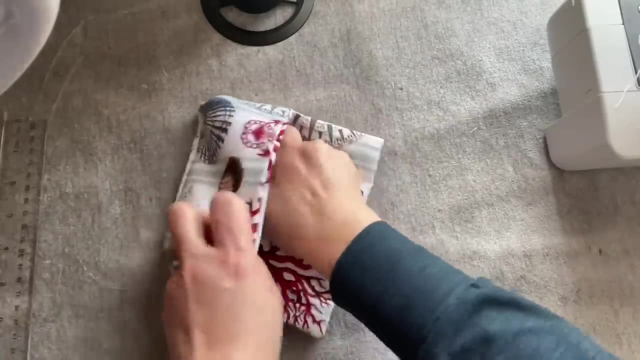 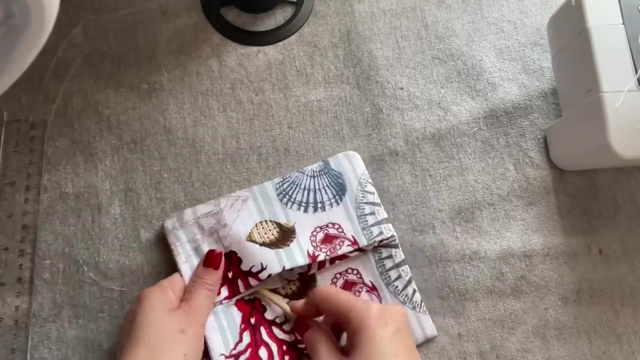 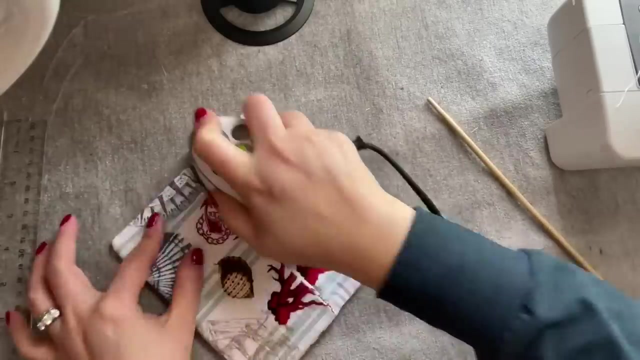 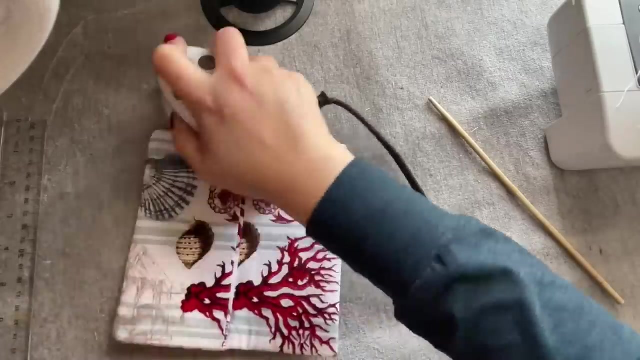 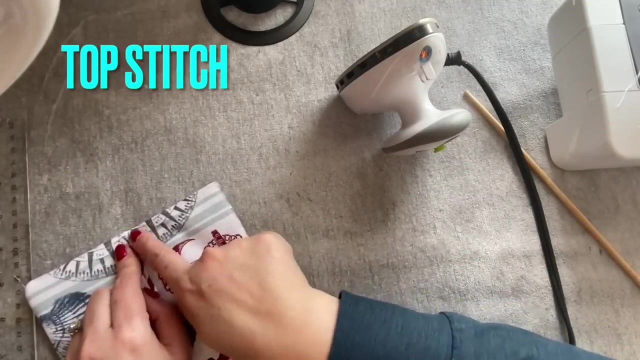 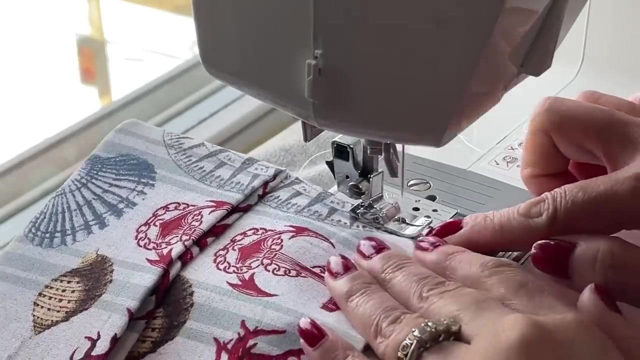 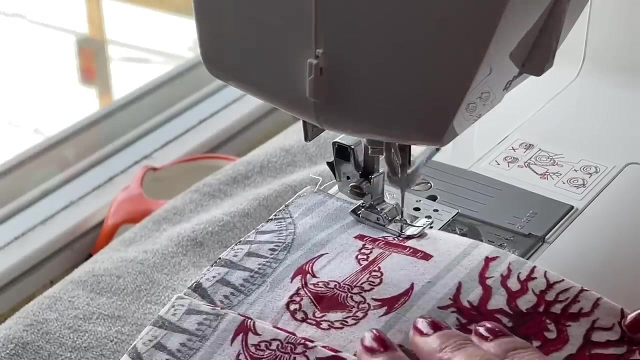 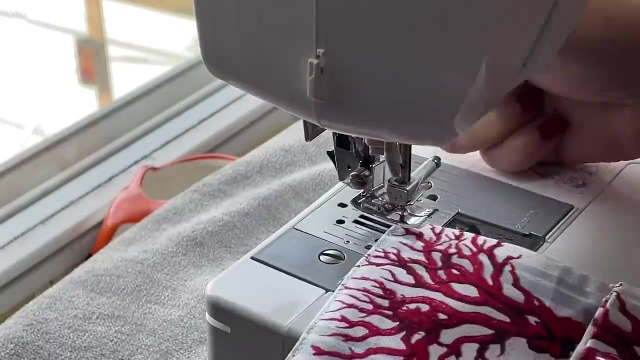 Push it in So it can stay on the bottom inside here. Now you're going to sew top, stitch just this part right here And go this way and go down to this way, And now we sew the other side, See. So all you do is Women closedối. 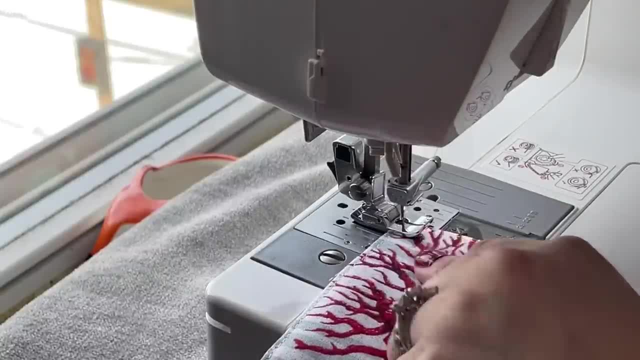 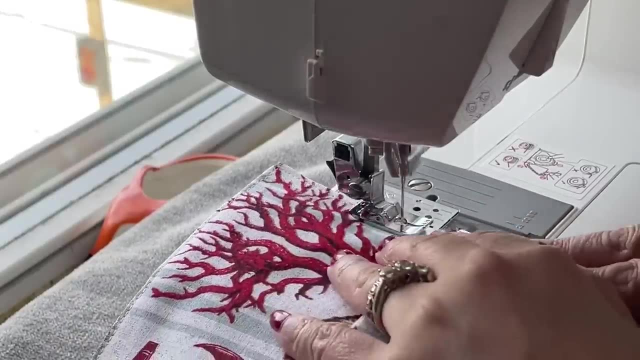 See, Co males go inside the center like this. So now, right here, lets go in, Push this And you can see. well, it went into the center So YOU can go down, you can line it, you know, whatever part you put into the socket. 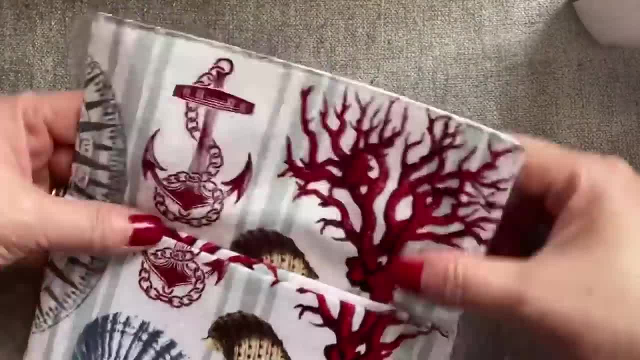 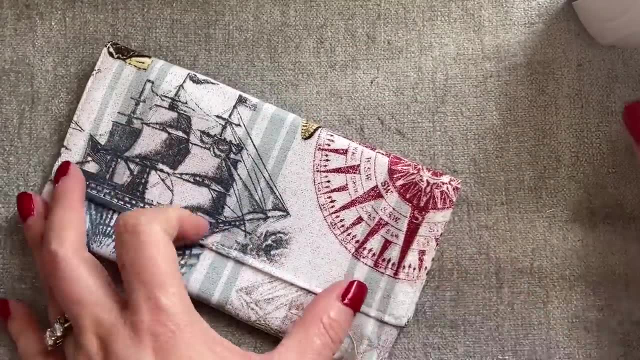 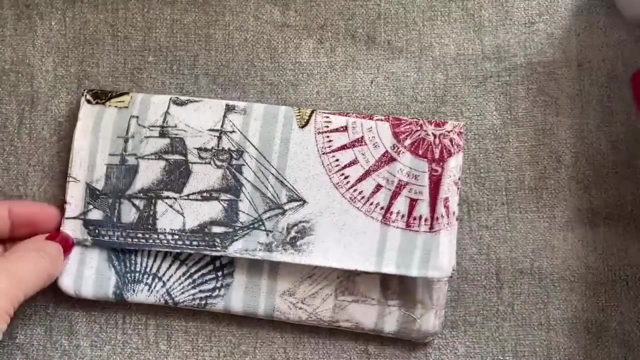 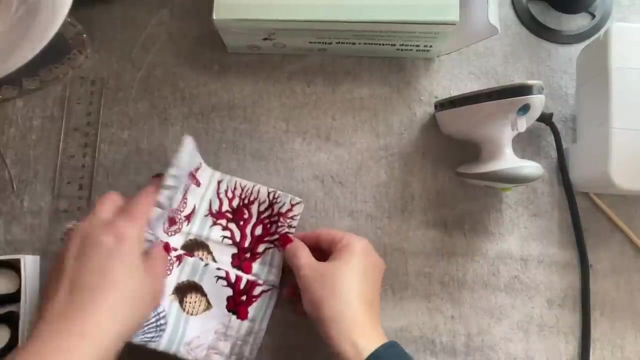 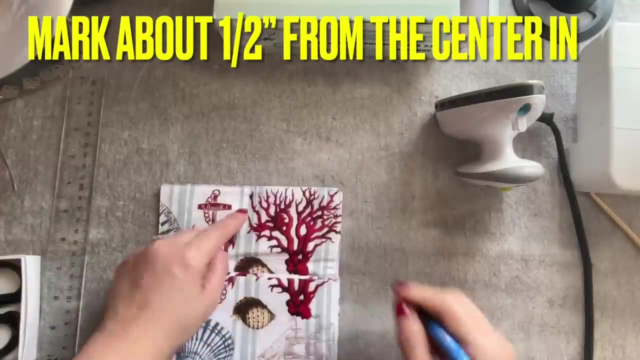 Now, when you're done, you're back inside the center. Thank you, Bye, Bye, Bye, Bye, Bye, Bye. okay, so now we're going to add the button to it, okay, so now I'm going to fold on the flap this way and I'm going to press enter. so about close to half an. 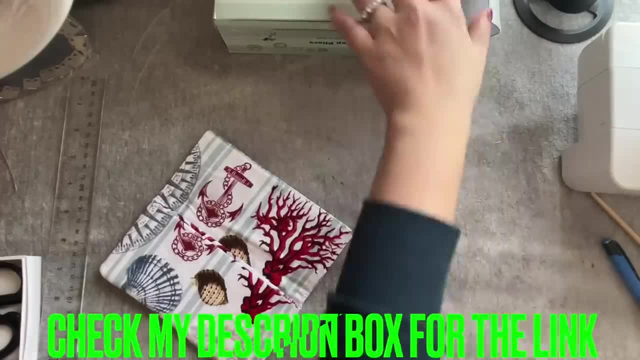 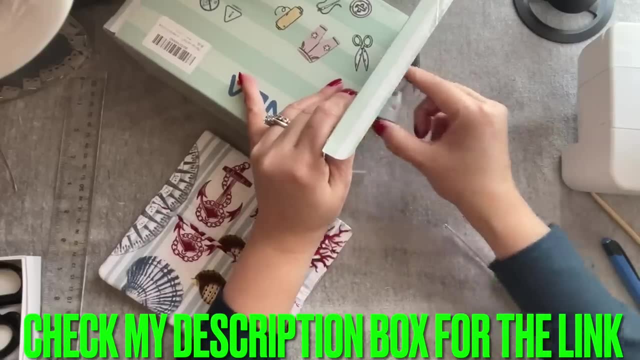 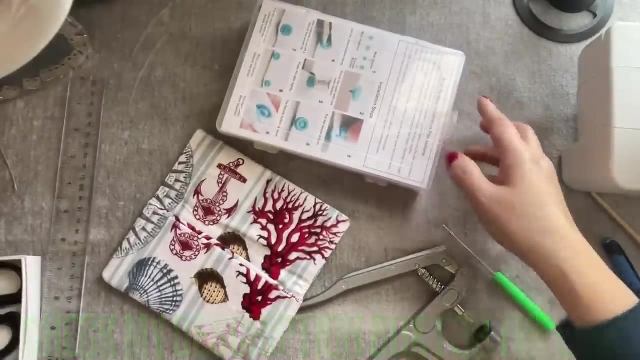 inch on the line that you mark right there. so I have the button that. I got it here everyone you can check in my description for the link. it's really, really good and it you can make so many. you never ran out of button. it come with so many thing in here, so 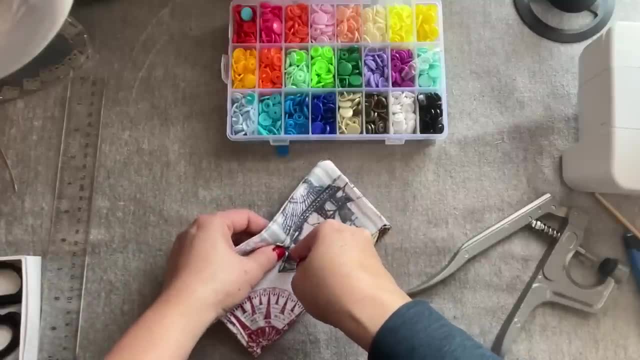 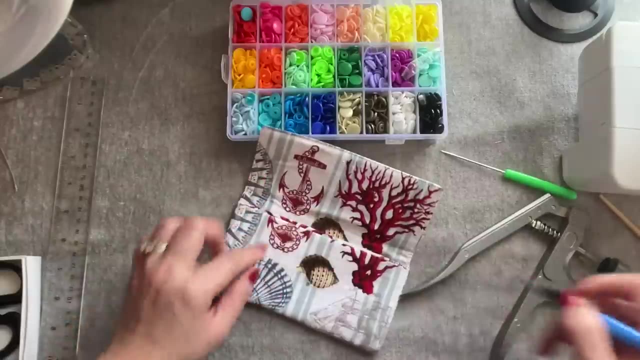 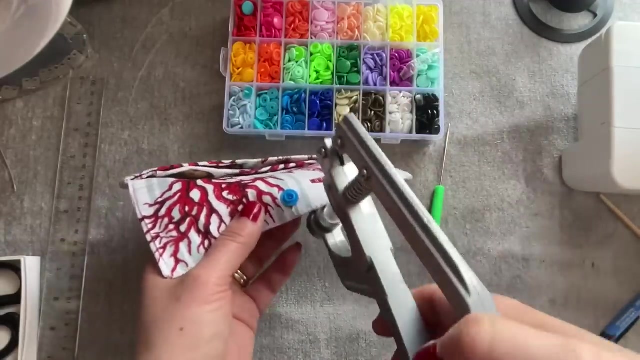 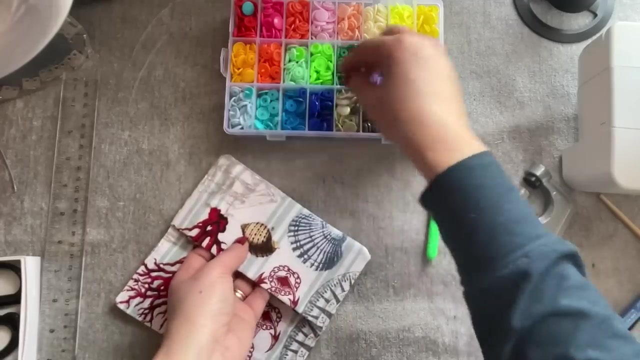 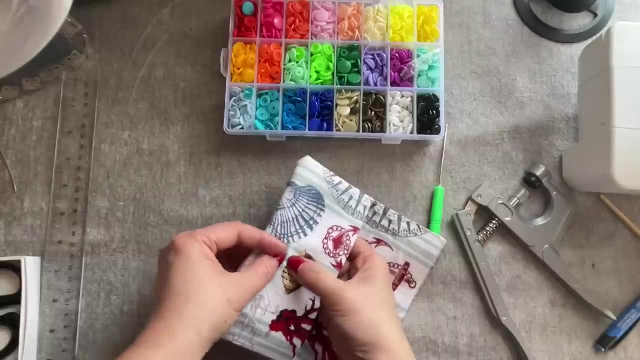 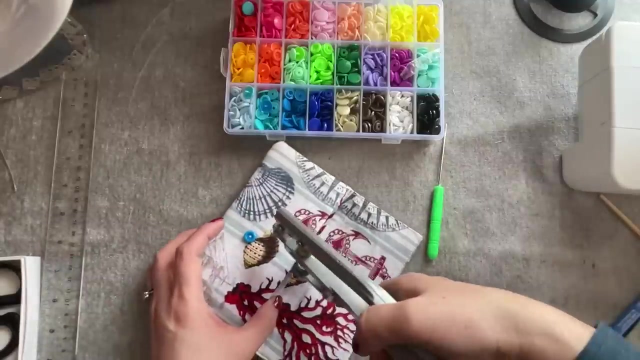 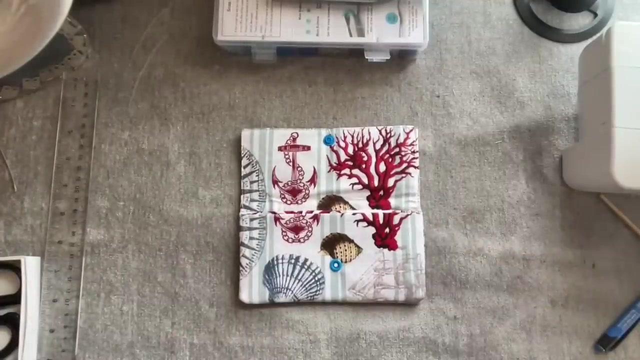 and you're going to poke through the other side too, so you can mark this other side like this, okay, so you're going to mark that line right there. you can take the regular buttons and this is the plan. okay, so this is the reference for the hole size, for this is the beginners guide. no, you can just. 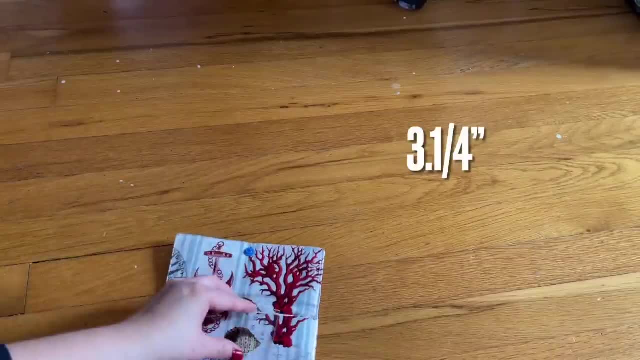 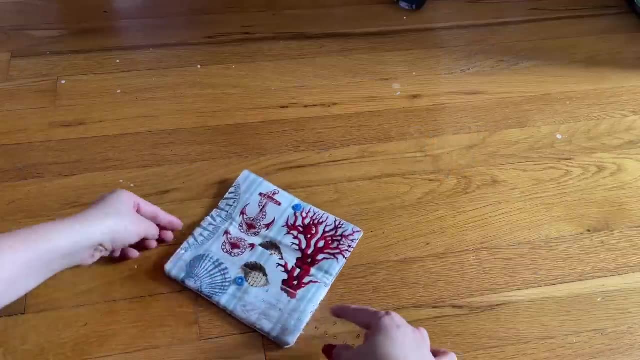 make the hole your own. and now I'm going to put in the buttons inside the pocket. it's the same that I did in the past, and so I'm going to make it so that you can not make a hole in it. that's the other side, and then I'm going to make a 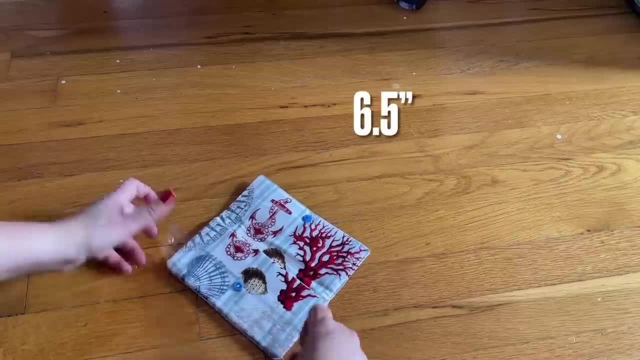 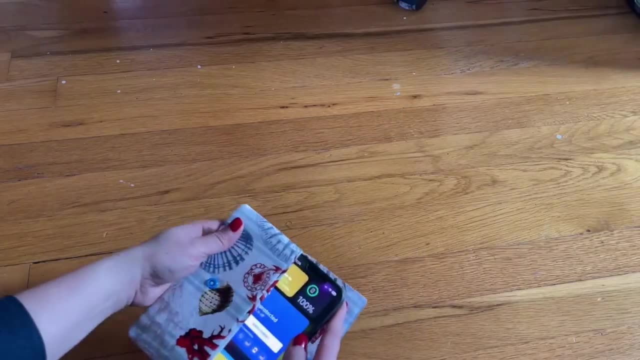 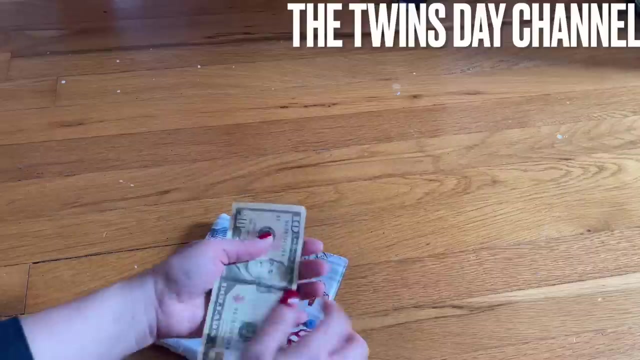 and then the wide side is six and a half so it can fit the phone. this is iphone 13. you can place it in here just like so, slide right in for you perfectly see, and then the money you can straight out, like this money, you can straight it, and then you can put it here too, or you can.